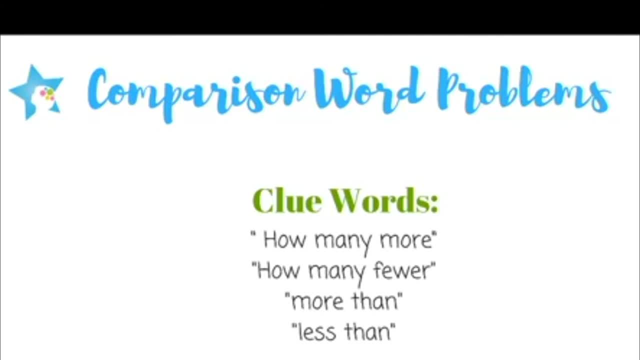 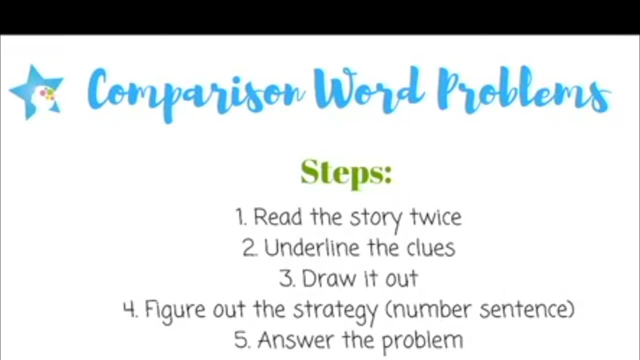 the word problem. there's a big possibility that this word problem is a comparison one. Okay, so what we're gonna do is we're gonna read the story twice. I have a couple of stories, a couple of word problems that we're going to go over. Then we're going to underline the 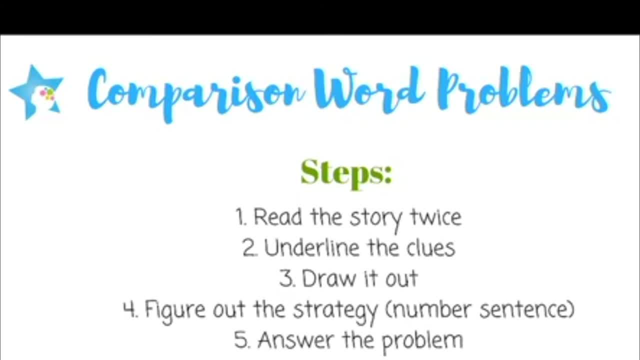 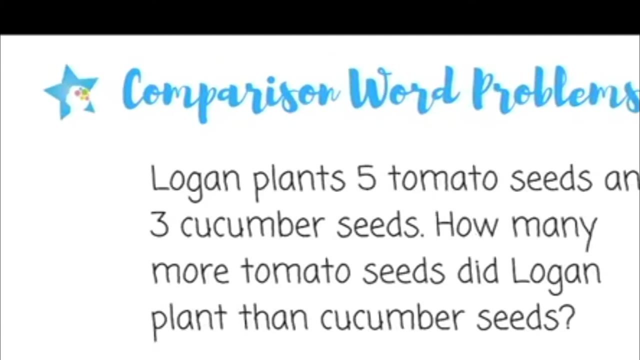 clues. We're going to draw it out, We're going to figure out a strategy. What number sentence would it be? Would it be addition or subtraction? And then we answer the problem. Okay, Um, so I'm going to go to my let's. let's look at the first one here, All right? So the first one says Logan. 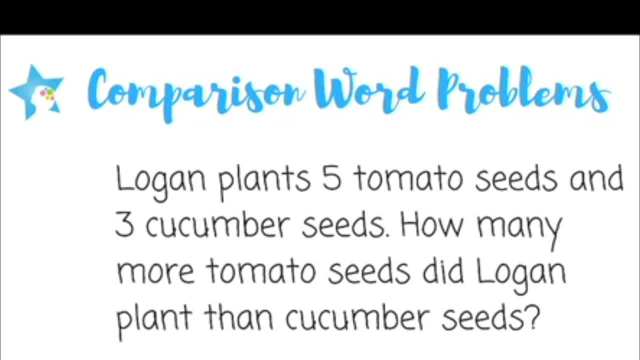 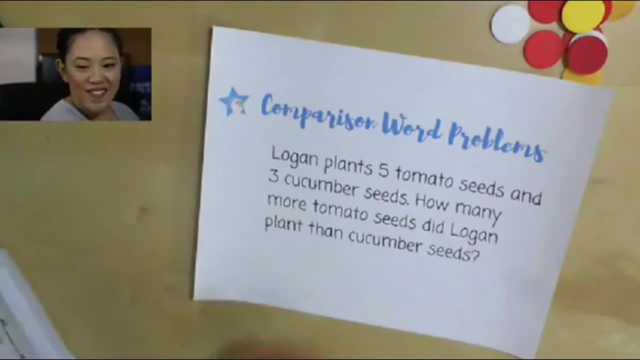 plants five tomato seeds and three cucumber seeds. How many more tomato seeds did Logan plant than cucumber seeds? All right, So let's take a look at this. Okay, So I have all these papers here. All right, Let's read it one more time. Logan plants five tomato seeds and three cucumber. 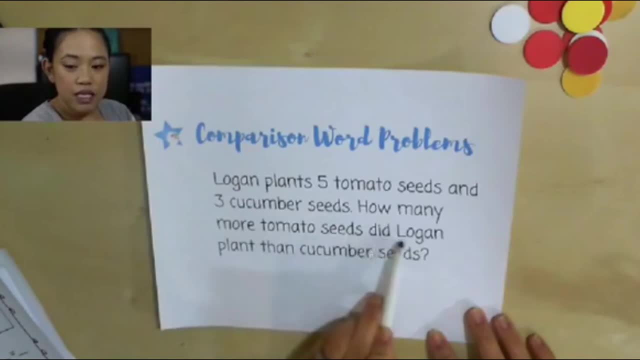 seeds. How many more tomato seeds did Logan plant than cucumber seeds? All right, So we're going to underline the clues. I know in word problems, um the the numbers that they write on there could be a really big clue. So I'm going to underline line five: tomato. 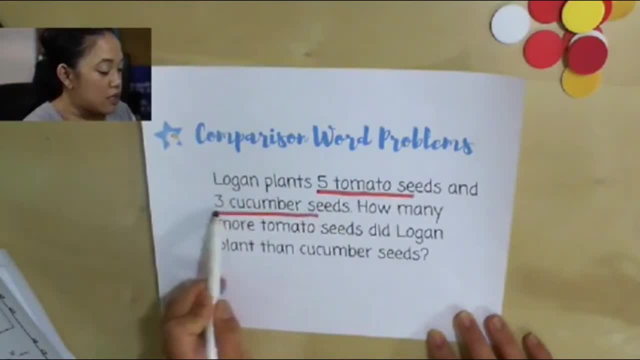 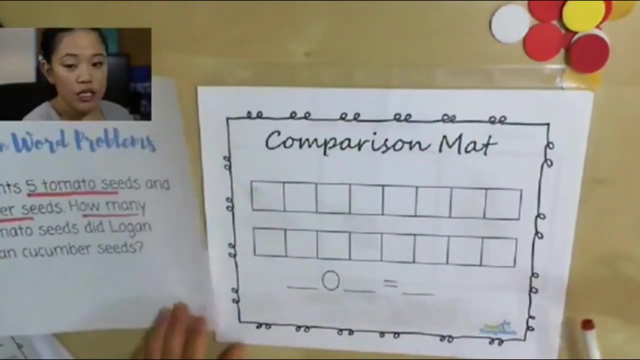 seeds. Oh, there's three cucumber seeds. And then it says how many more? how many more? That's a comparison story problem. It's a comparison, Comparison word problems. So I'm going to grab my comparison mat here and I'm going to use the 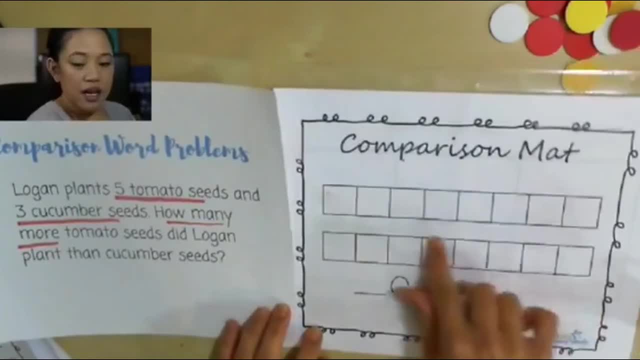 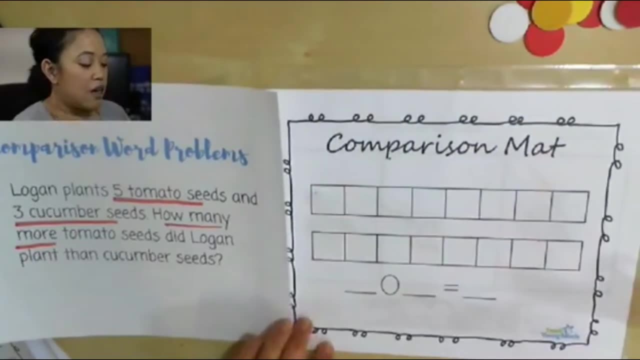 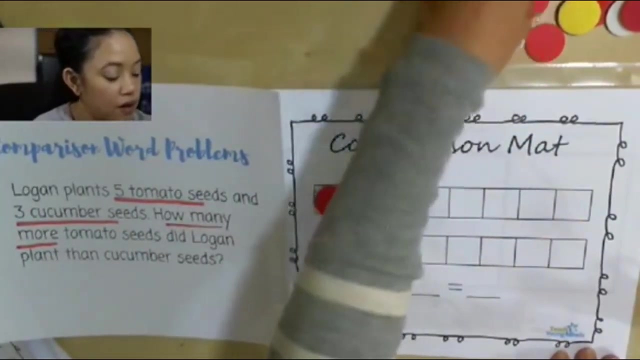 clues to help me, kind of, um, draw this out, We're not going to draw it out, I'm going to use these counters here. Okay, All right? Um, I have five tomato seeds, so I'm going to make these five here, Three, four. 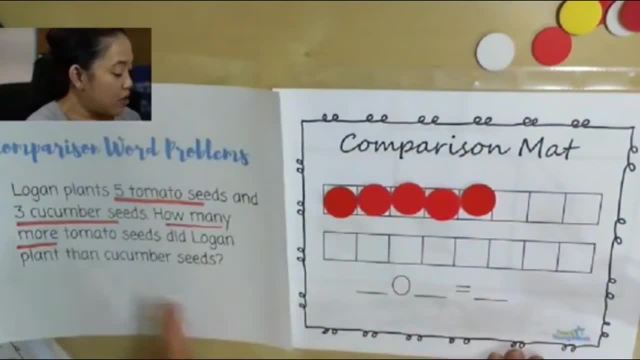 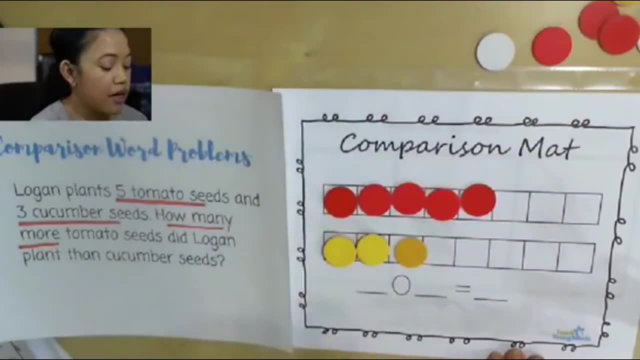 five and three cucumber seeds, And I'll do cucumber seeds in this color, All right. Now, when we compare, really what we're doing is we're seeing how many more, how many extra, or how many fewer, how many are missing. Um, and this is asking: how many more? 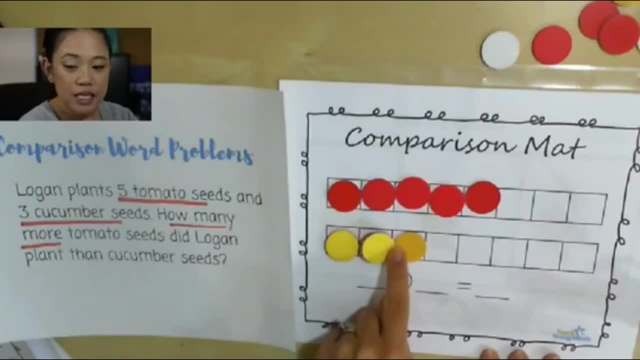 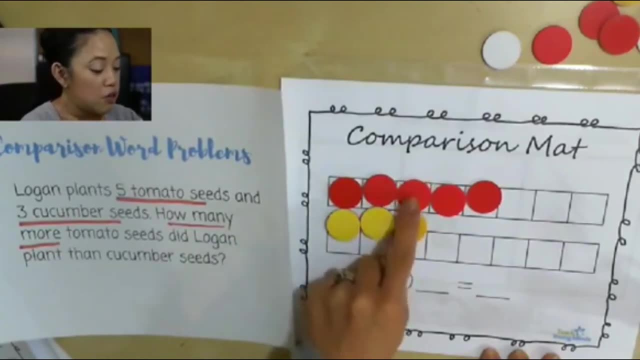 So we want to know how many more tomato seeds there are than than cucumber seeds. So what I like to do is I like to match them up. I'm going to push those together And how many more tomato seeds are over there? How many extra are there? There's two. 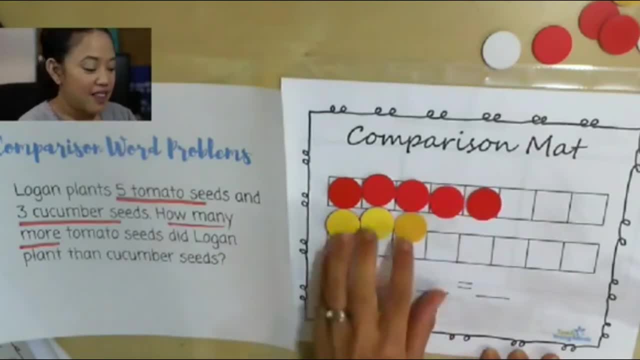 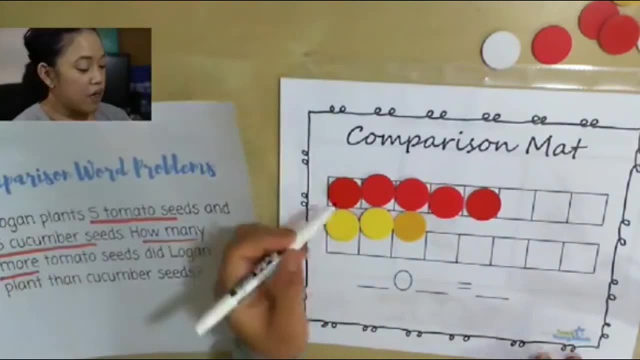 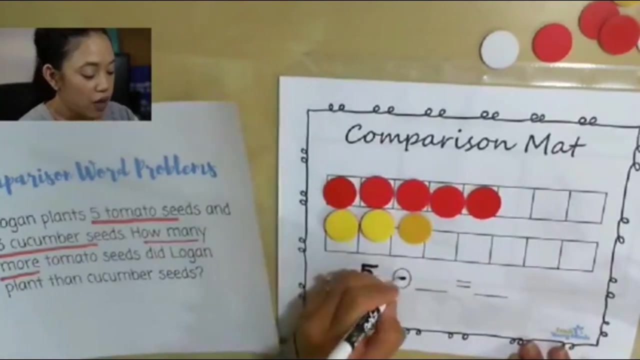 there's two extra tomato seeds- Okay. So what we can say in this story problem is- I'm looking for my marker here. There's five tomato seeds, taking away the ones that have a match. Okay, So we're taking away the three and there's two left over, Right, So we can say that there. 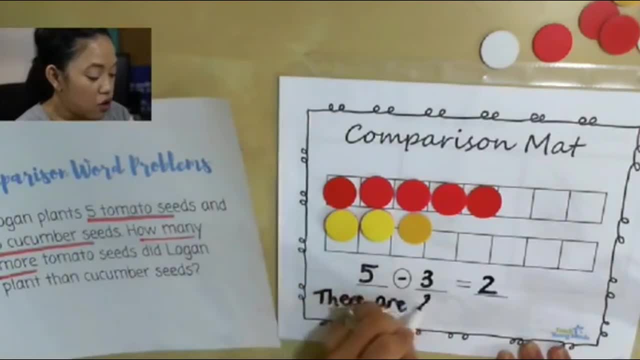 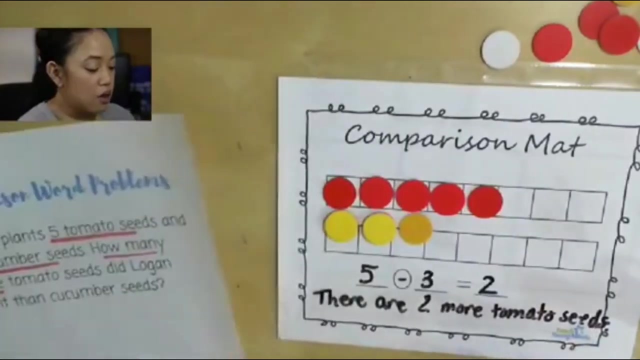 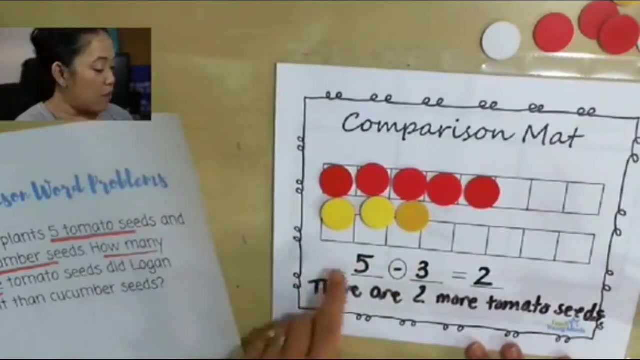 are two more tomato seeds Right. So we read the story twice, We underlined the keywords, We drew it out or we used um tools, math tools, to help us. Then we figure it out, The strategy we decided we were going to. 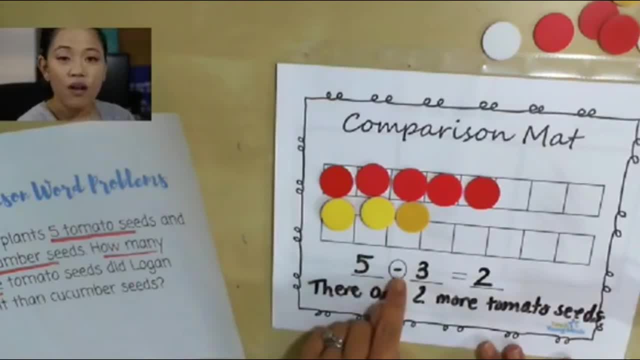 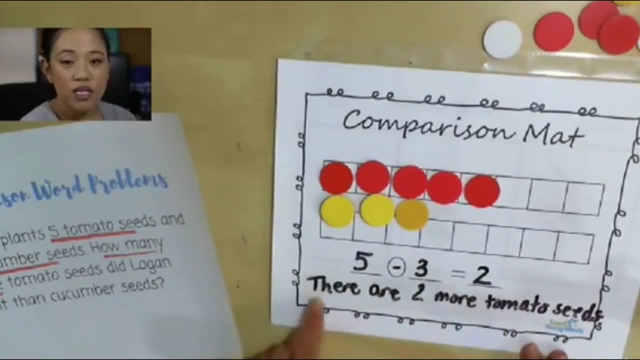 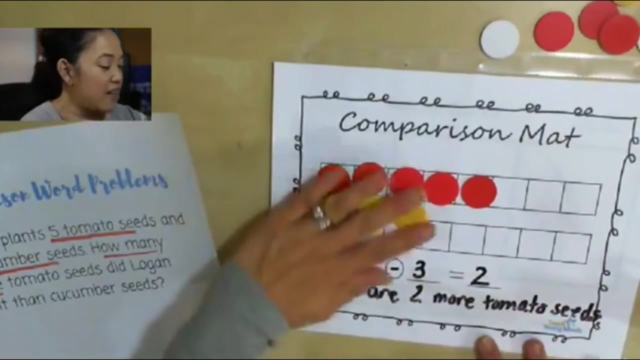 do subtraction. That's one of the ways That's what we're um practicing today. We're doing the subtraction strategy for comparison word problems And then we wrote the answer at the bottom. We finished the answer. There are two more tomato seeds. Okay, Let's try another one. 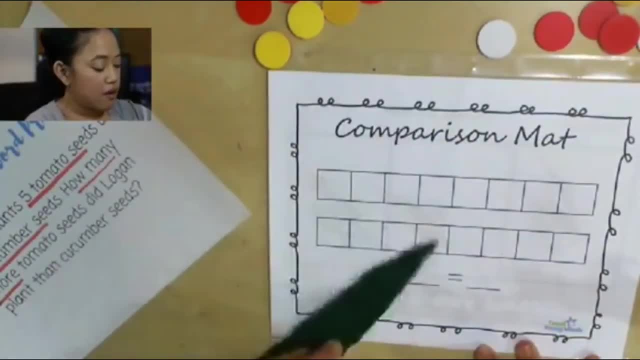 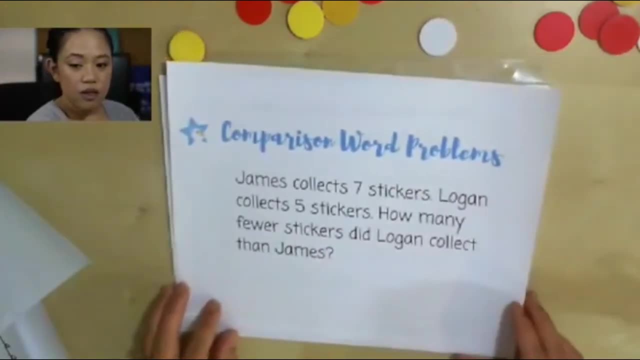 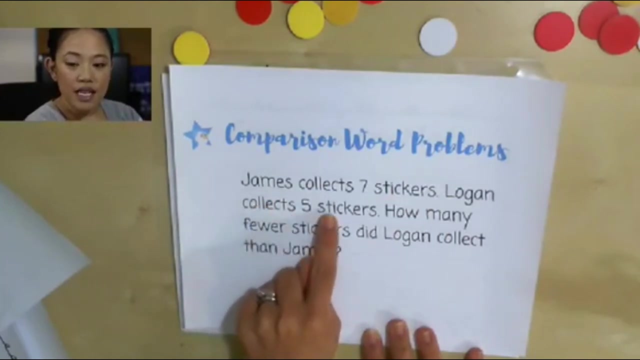 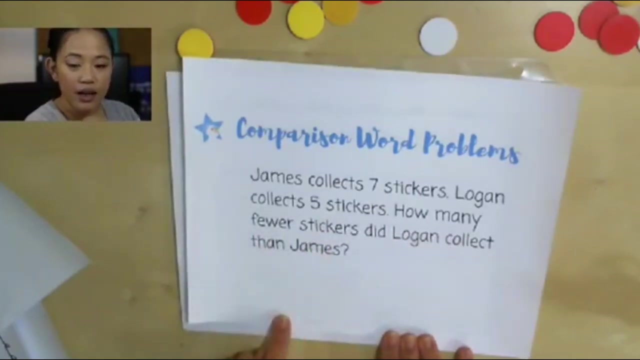 Erase this. All right, Let's go for the next one. Let me find the next one, Okay. So here's the next one for us. James collects seven stickers. Logan collects five stickers. How many fewer stickers did Logan collect than James? Let's read that one more time. James collects seven stickers. 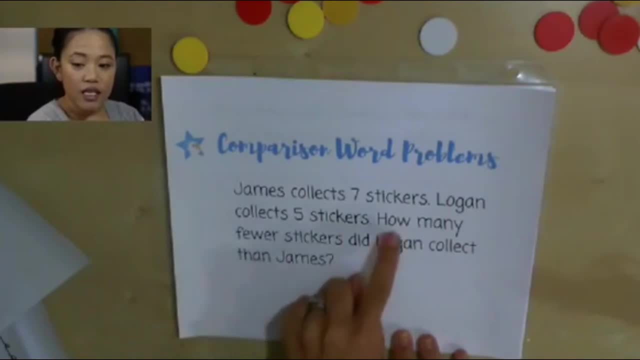 Logan collects five stickers. How many fewer stickers did Logan collect than James? So what do we do next? We've read the story twice. We read the word problem twice. Now we underline the clues. All right, So James collects seven stickers. Logan collects five stickers. How many? 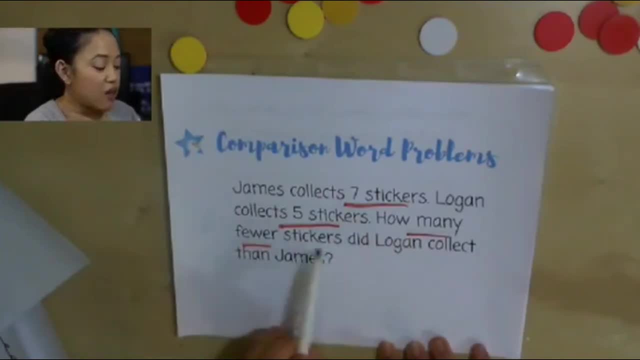 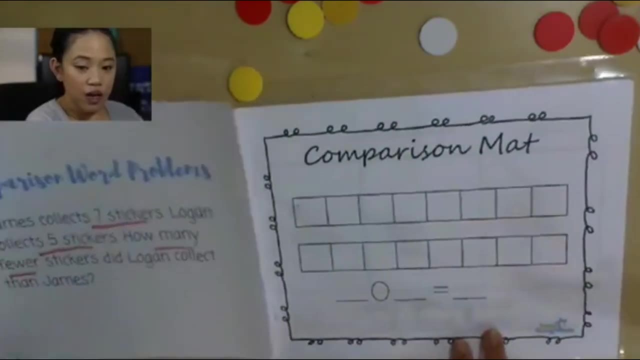 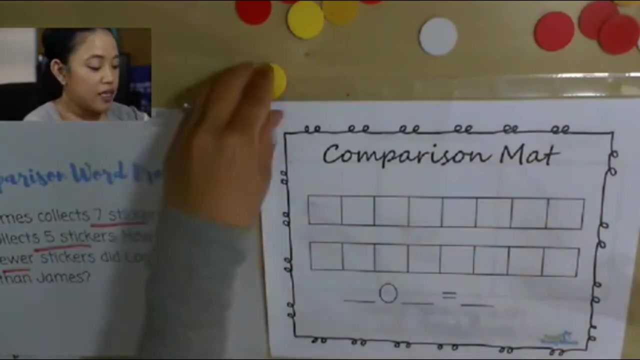 fewer stickers there are. That clue tells us that it's a comparison word problem. All right, so let's go to our board and let's draw it out. Okay, this time in instead of using um. this time, instead of using the counters- how we push them together, I'm gonna use um. I'm just gonna draw it out, All right. 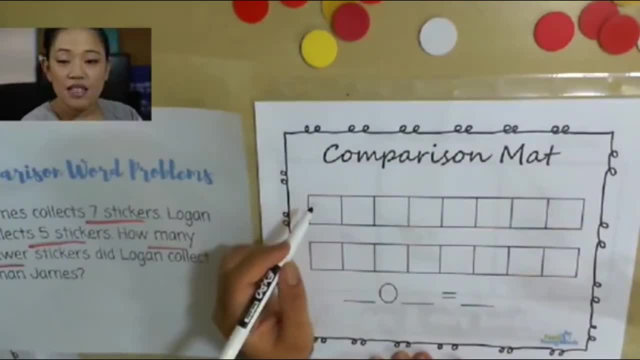 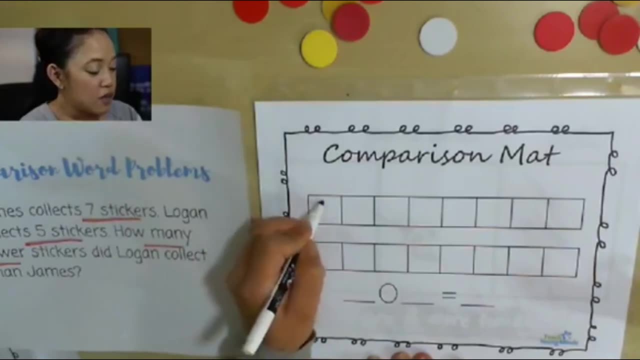 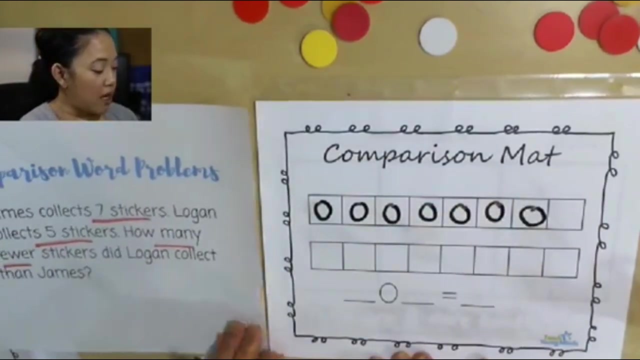 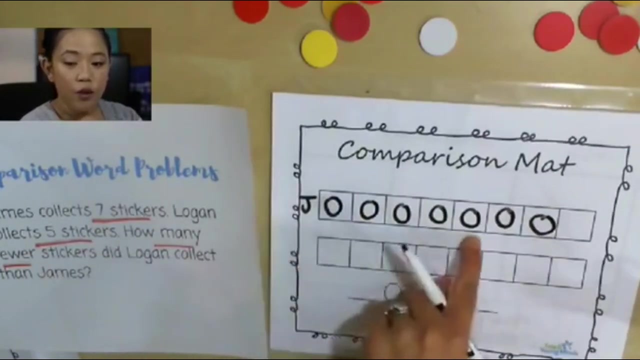 okay, So James collects seven stickers. The fastest way for us to do it is just to do circles. Okay, seven stickers: One, two, three, four, five, six, seven. Now how many? now that we have James, I like to label to show um who has what. Now we have to find out Logan, How many? 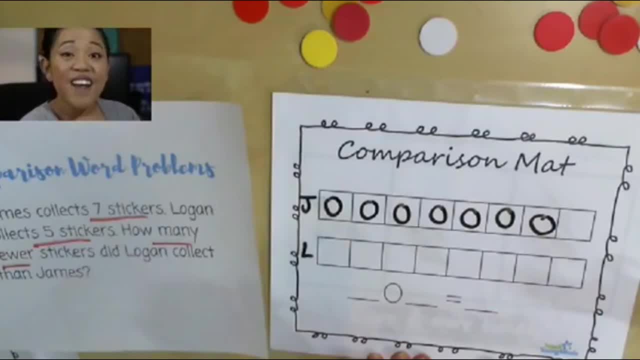 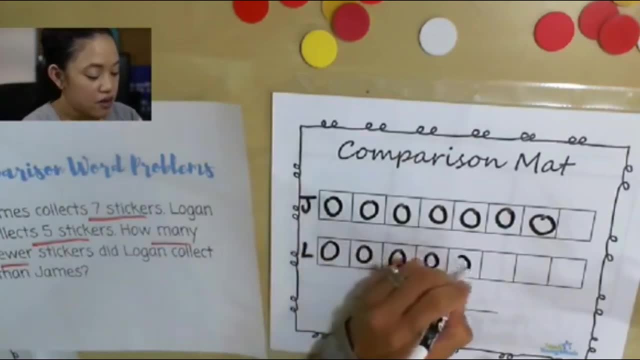 stickers. does he have? Logan have Five. So what are we going to draw here? Five circles right, One, two, three, four, five. Now the next thing we do when we do comparison: remember, we match these up, Remember. 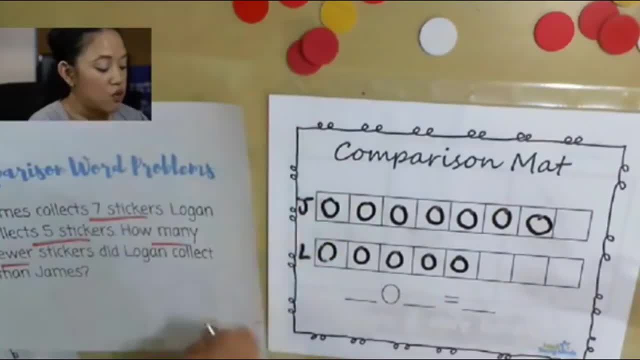 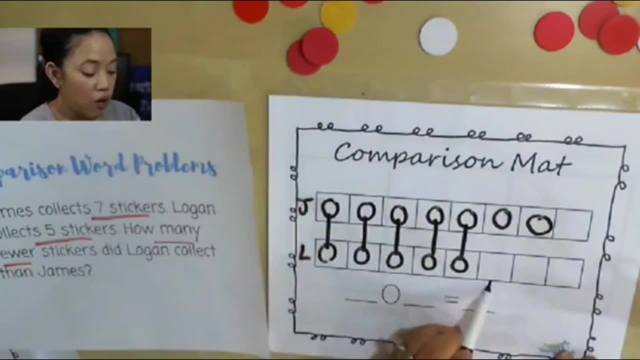 when we match them up. all I'm going to do is draw a matching line. I'm going to match them up. Oh, how many are missing here? Logan is missing two. or Logan has two fewer stickers than James. Logan has two fewer stickers than James. Okay, so let's write the story. See if you can try it. 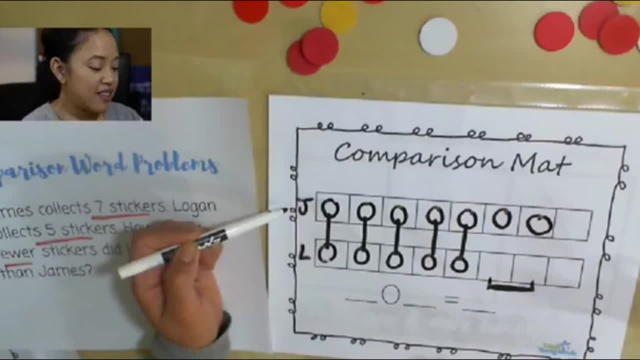 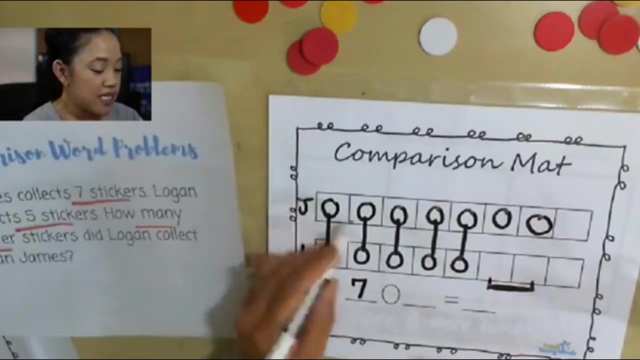 Write down how much James has, Then write down how much Logan has, how many stickers Logan has. Are we adding or subtracting here And then get your answer. Okay, friends, let's check your work. So there's seven. James has seven stickers, Logan has five. 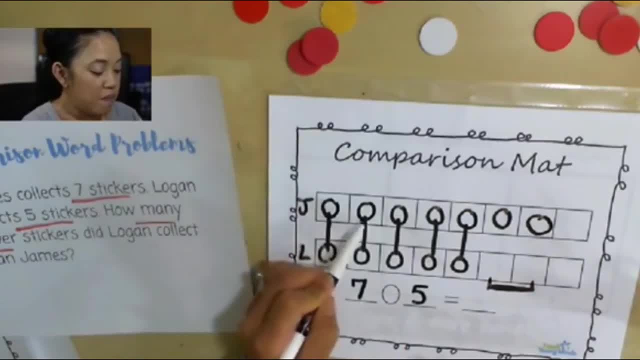 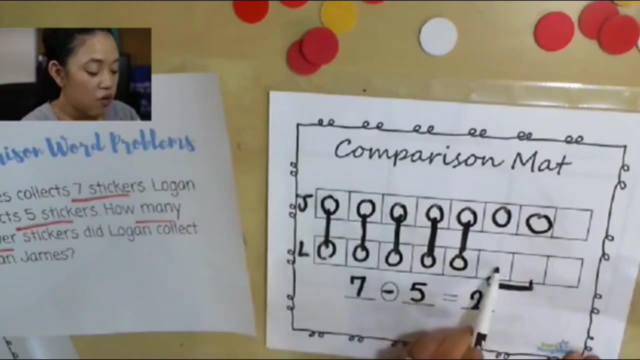 And we are matching up the ones that have a partner, I like to say: So that's subtraction. And then we have two left over or two missing. So we can say Logan has two fewer stickers than James. So that's subtraction. And then we have two left over or two missing. So we can say Logan has two fewer stickers than James. 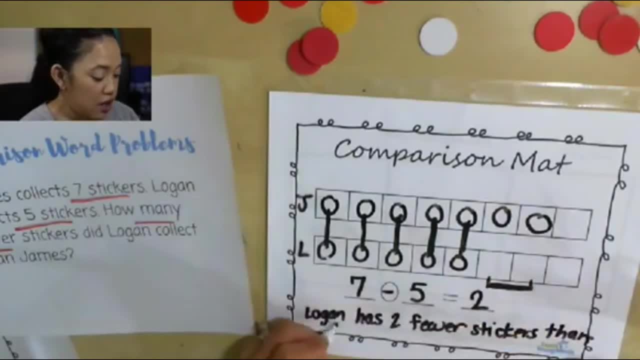 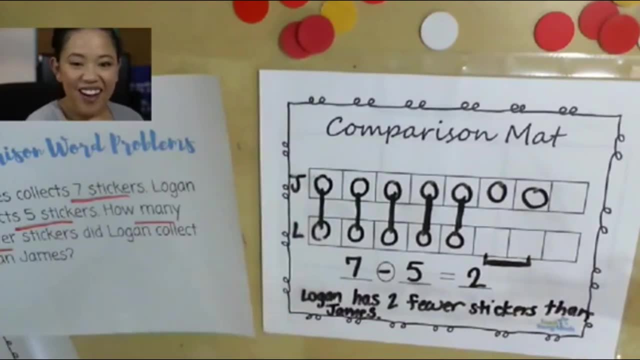 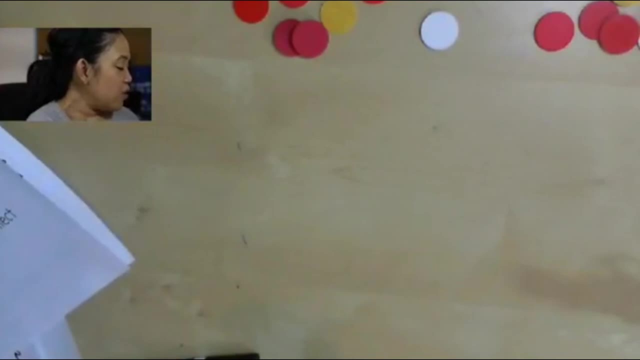 So that's subtraction. And then we have two fewer stickers than James. Okay, Alright, nice job, my friends. Okay, now we're going to get into the worksheet And you can use your counters still, But I'm going to draw mine out. 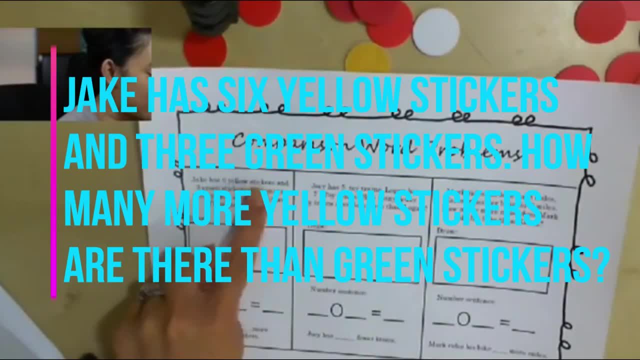 Okay, Jake has six yellow stickers and three green stickers, And you can use your counter still, but I'm going to draw mine out. Okay, Jake has six yellow stickers and three green stickers. How many more yellow stickers are there than green stickers? 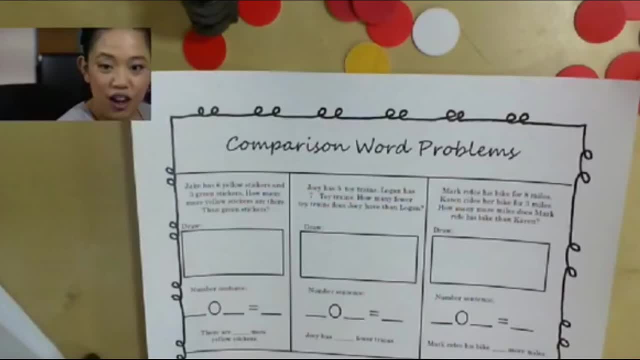 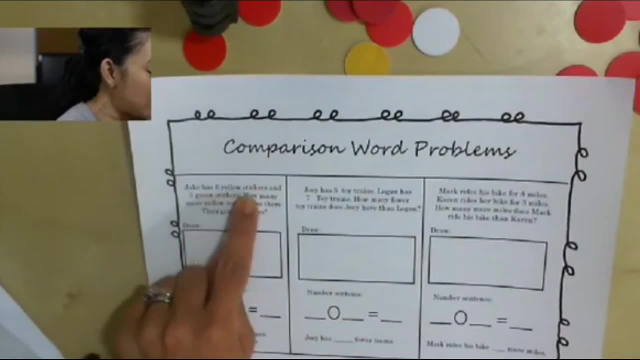 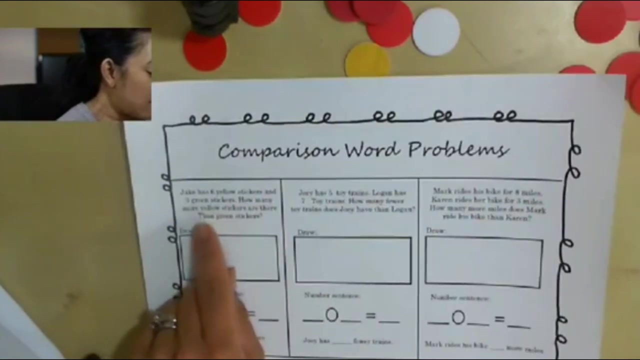 All right, so let's- ooh, I was about to draw it out, but we don't do that yet. We're going to read it one more time and underline the clues. Jake has three yellow stickers and three green stickers. How many more yellow stickers are there than green stickers? 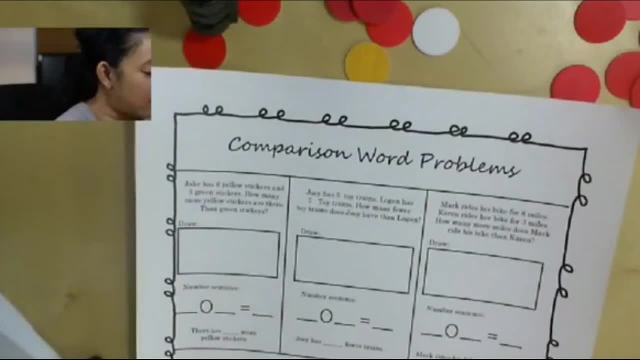 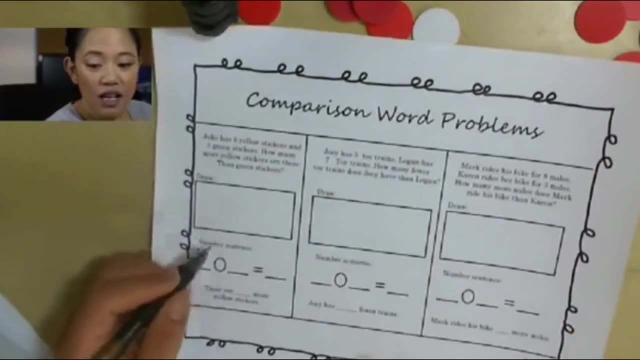 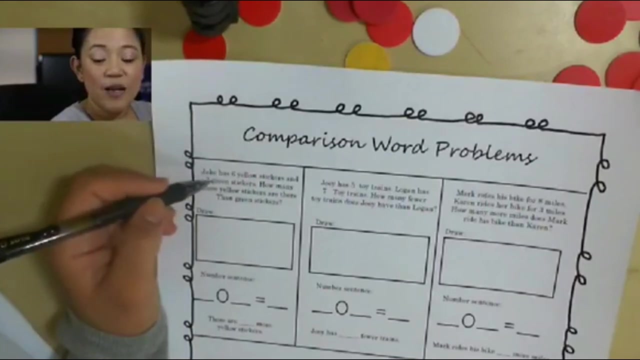 So now we're going to underline the clues, and normally we use a pencil in math, but just so that you can see better on here, I'm going to do a pen, okay, So go ahead, let's see which ones are the clues. 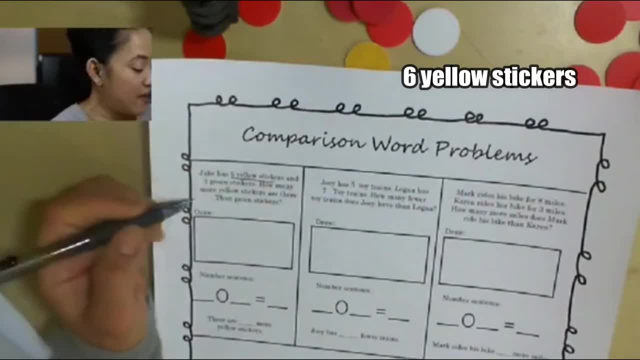 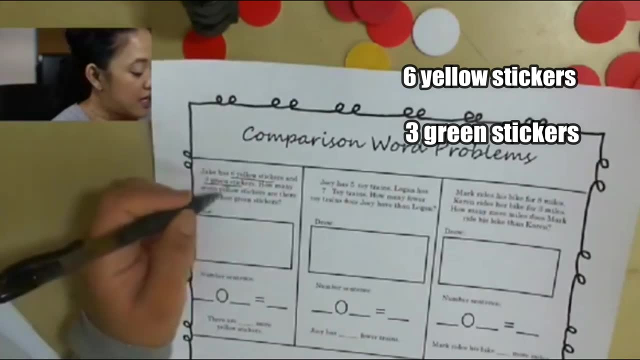 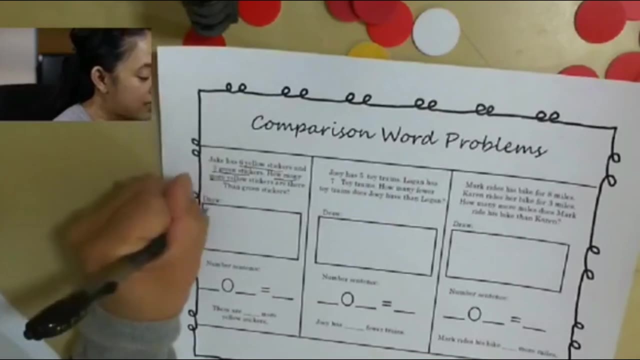 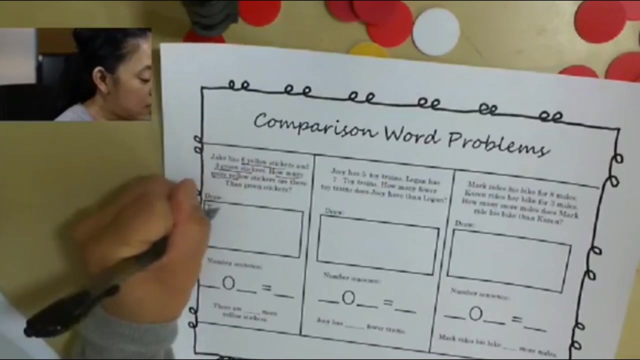 Six yellow stickers and three green stickers, And then it's asking how many more? so we know that's a comparison. okay, Let's draw this out. There's Jake J for Jake, and I'm going to do six yellow stickers. 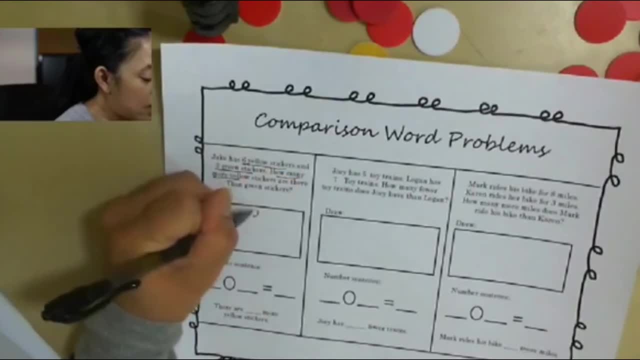 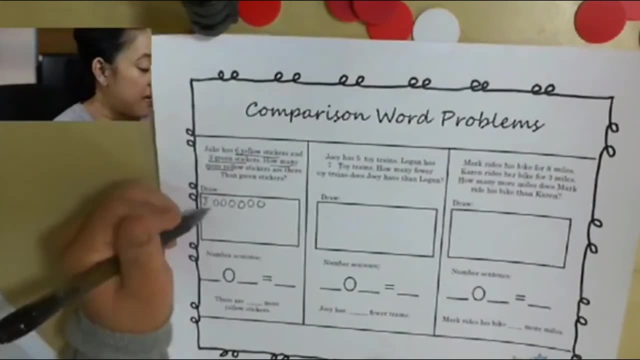 I'm going to draw six circles, and it's. we want to try to be nice and neat In math. it's important that we're neat with our work because otherwise we'd make a mistake. right, Okay, Okay, It's a lot easier for us to make mistakes. 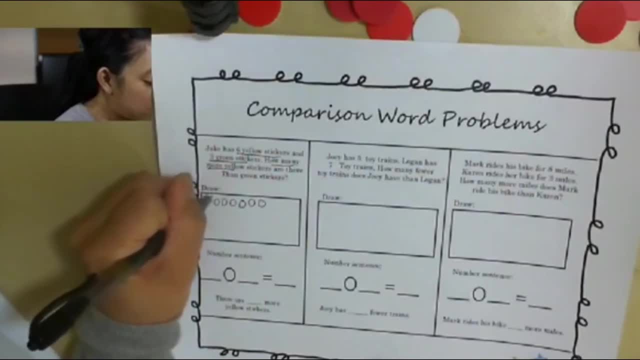 Oh, actually this means yellow. See, I already made one mistake. That's okay, no big deal. And this one's green, G for green and there's three green stickers. Okay, my friends, now what do we do? 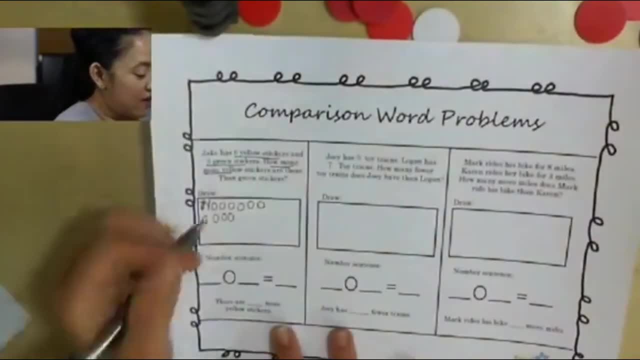 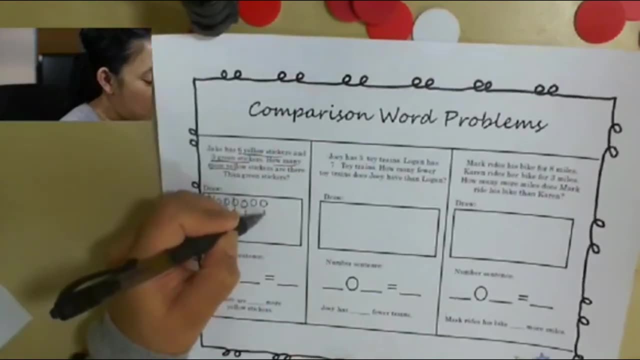 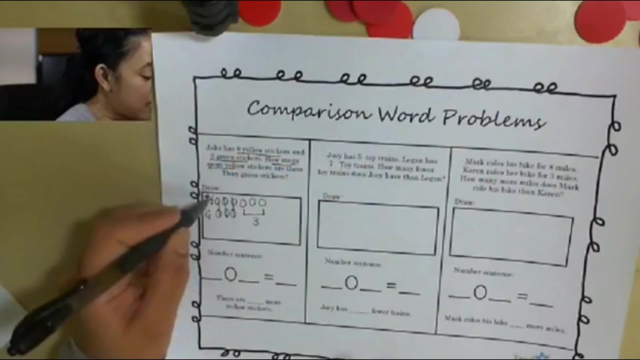 We match them up, just like in the last one, because we know it's a comparison. We match them up and now this tells us how many we have left over and it looks like there's three there. So our story problem is yellow stickers. there's six and there's three green stickers. 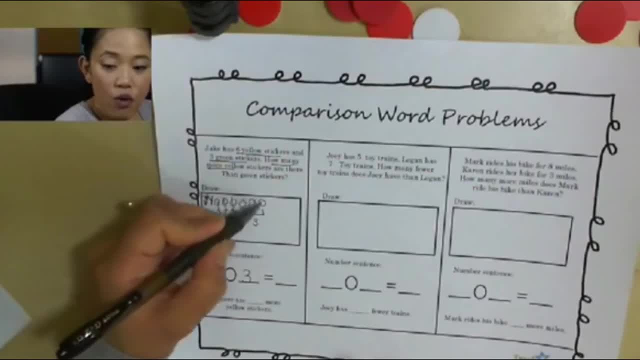 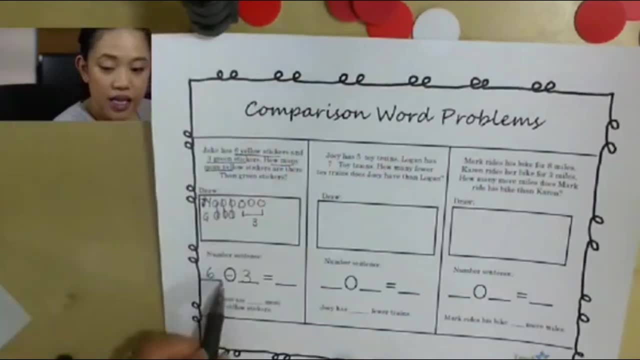 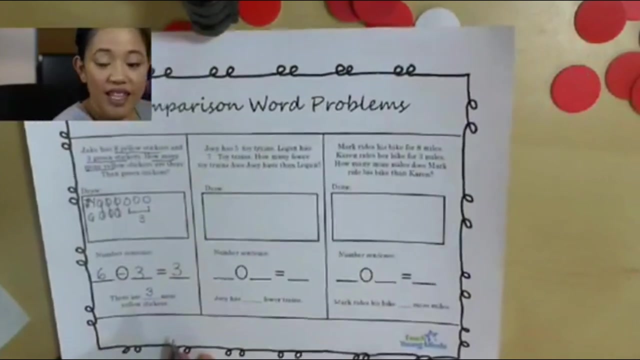 We match them up and we're only looking at the extra. okay, So we're taking away the ones that have partners, and that equals three. There are three more yellow stickers. All right, let's try this one, this one, this last one for today. 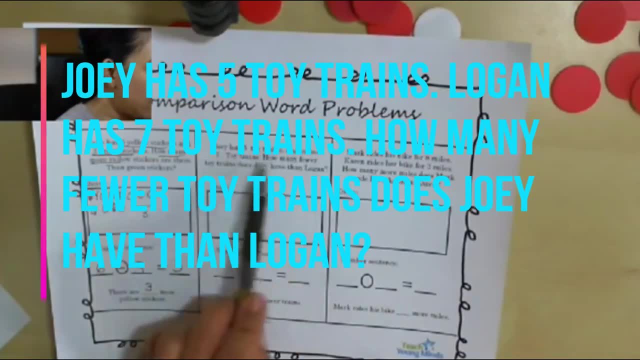 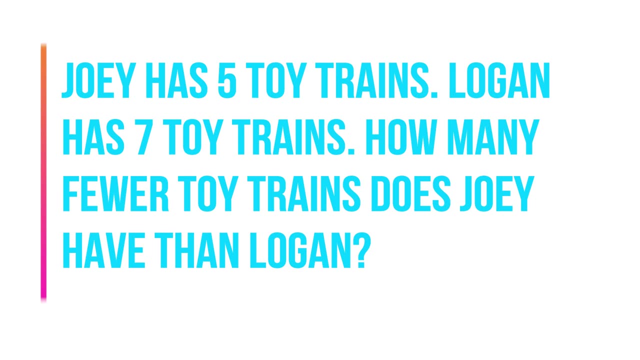 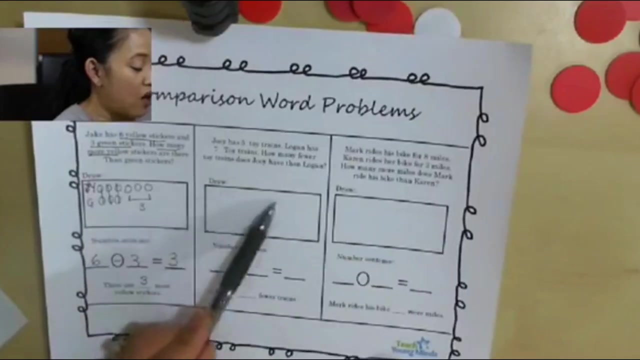 Joey has five toy trains. Logan has seven toy trains. How many fewer toy trains does Joey have? Okay, And then Logan. Okay. so this time I'm going to just give you a few minutes to draw it out, just like what I did here. 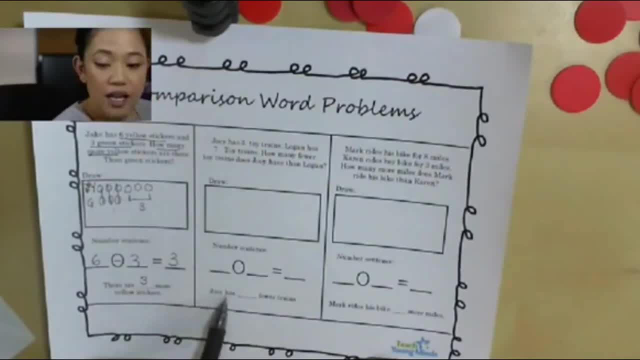 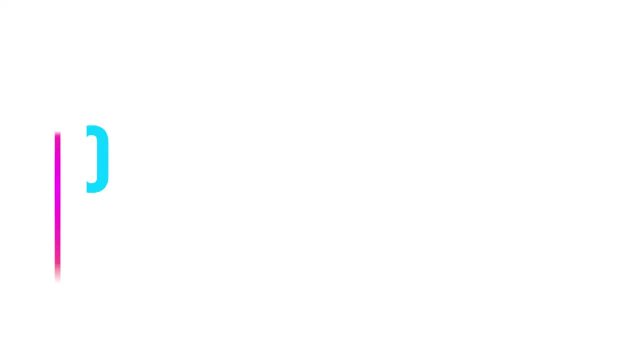 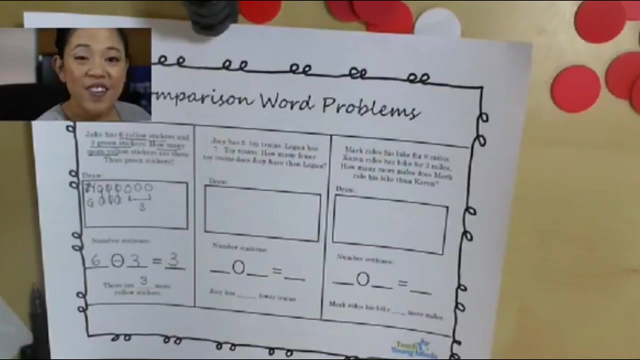 Then you're going to write the number sentence and then finish answering the word problem at the bottom. So I'm just going to give you a few minutes to do that. Okay, my friends, are you ready to check your answer Or are you ready to check your work? 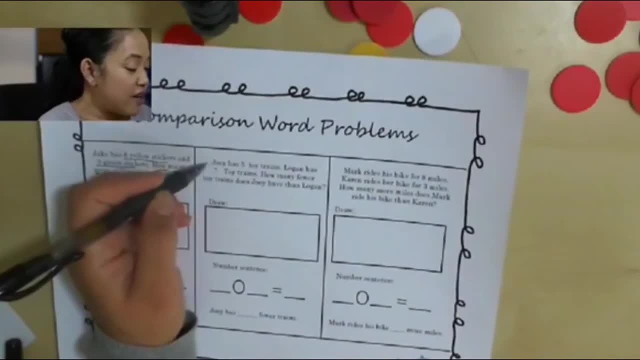 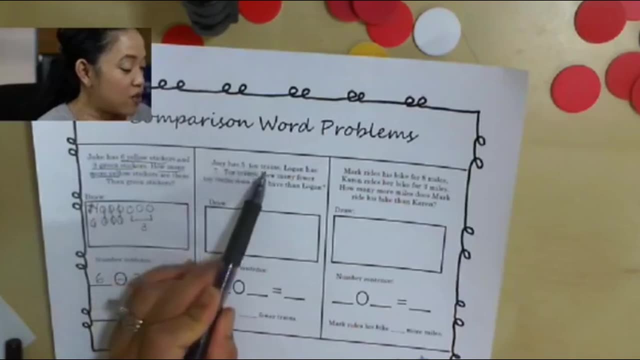 We'll get to the answer, but let's check our work first. All right, so we read the story. Let's read it one more time. Joey has five toy trains. Logan has seven toy trains. How many fewer toy trains does Joey have than Logan? 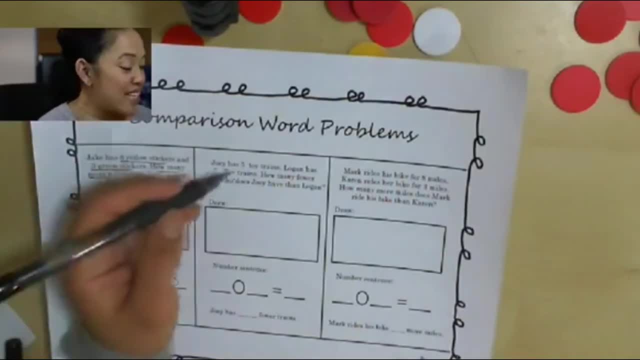 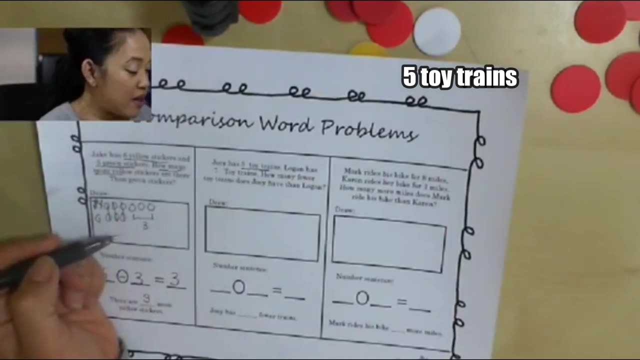 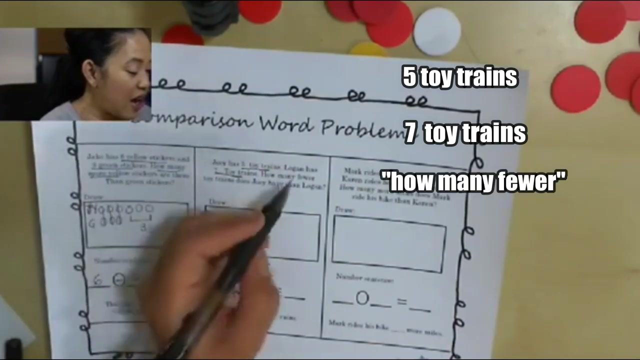 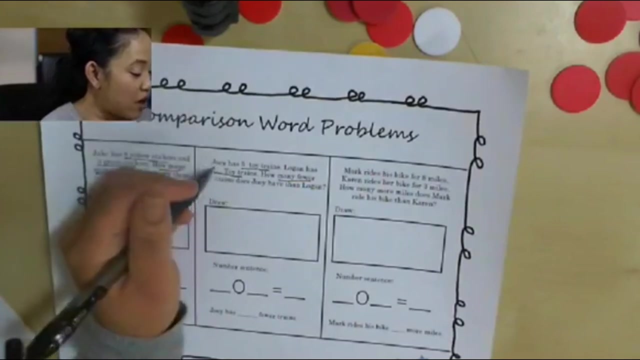 We read it twice. Now we're going to underline the key words, the key clues. There's five toy trains And seven toy trains. How many fewer? Those are the clues. All right, So now we're going to draw it out. 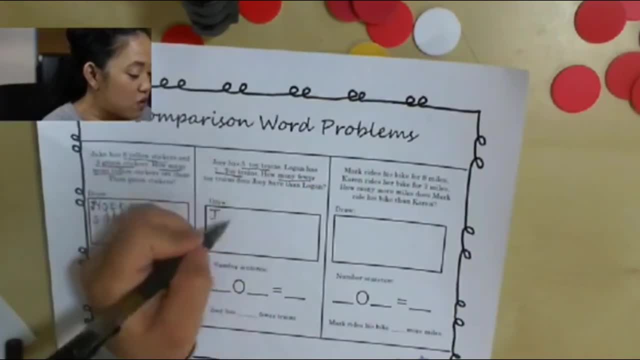 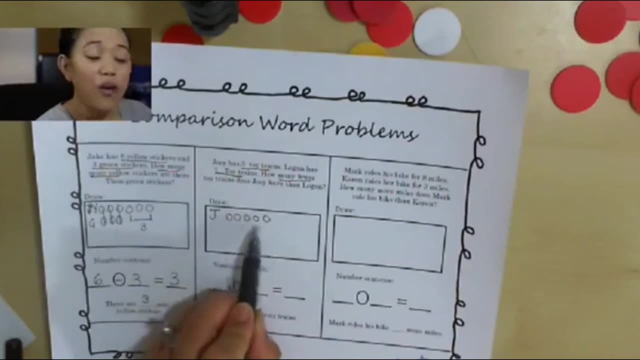 Joey J, for Joey has five toy trains: One, two, three, four, five. And remember we are just drawing circles because they're quick. We don't need to be drawing doodling little trains. That takes way too long. 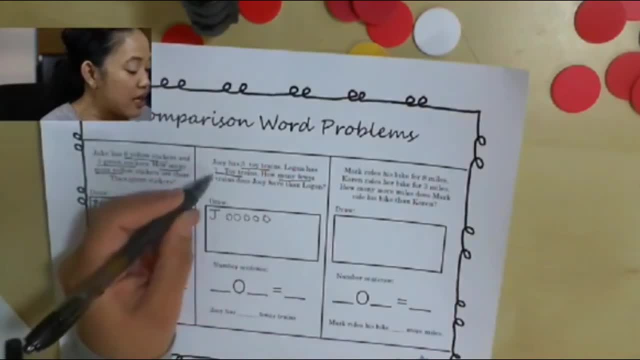 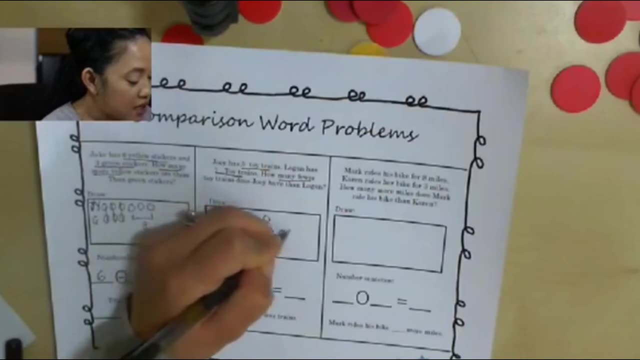 We like to be nice and simple, so we can get to the answer. okay, Logan, alpha, Logan- has seven: One, two, three, four, five, six, seven, And then, after we draw that, it says how many fewer. 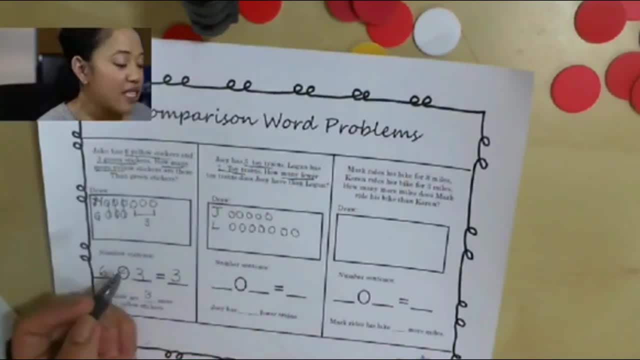 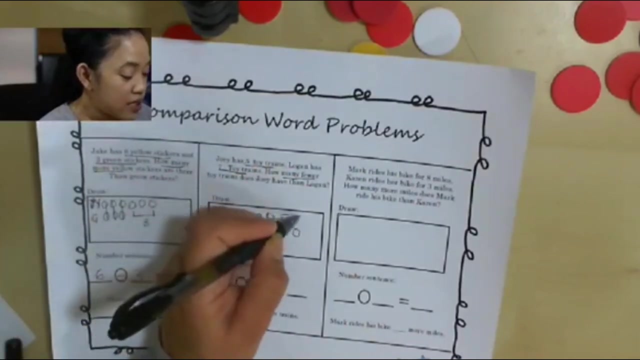 That's a clue, That it's a comparison, And when we compare we like to match them up right. All right, So we matched up. And how many fewer? looks like? Joey has two fewer, two missing here, So seven. 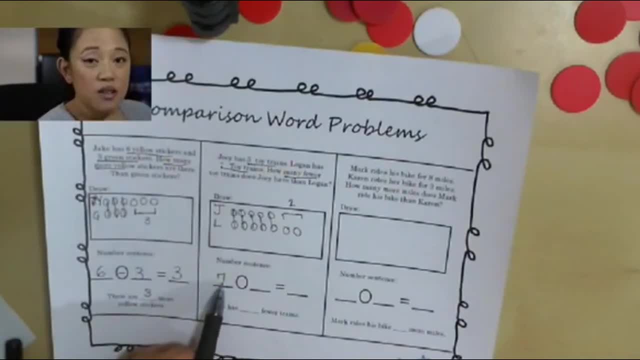 And the bigger number always starts the subtraction problem. I was really tempted to write five here, But seven. Seven is bigger than five, So we have to put the bigger number first in subtraction, okay, Otherwise it doesn't make sense, Or actually we can't do that.